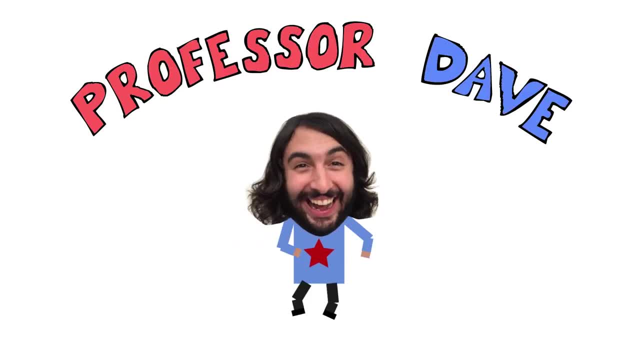 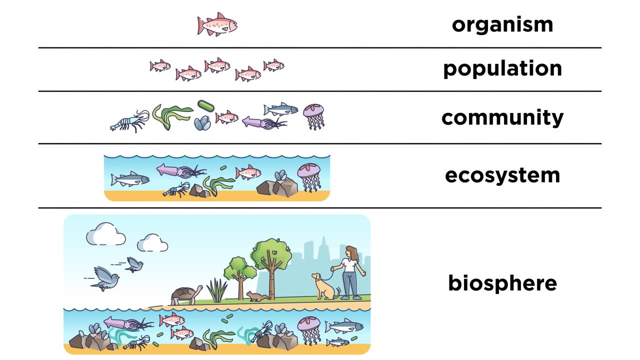 In the introduction to this series, we looked at all the tiers of complexity that an ecologist may study, starting with an individual organism and zooming out to consider the entire biosphere. Let's now take a closer look at all of these tiers, one at a time, so that we can get a better 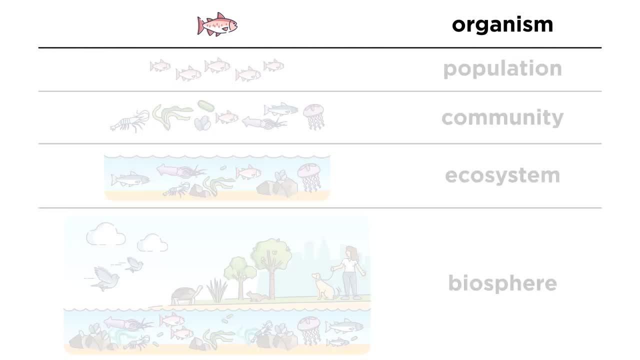 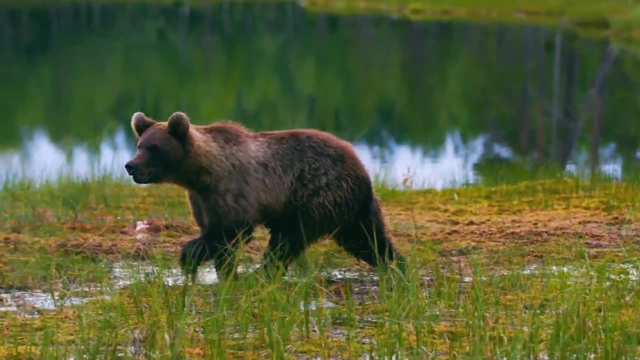 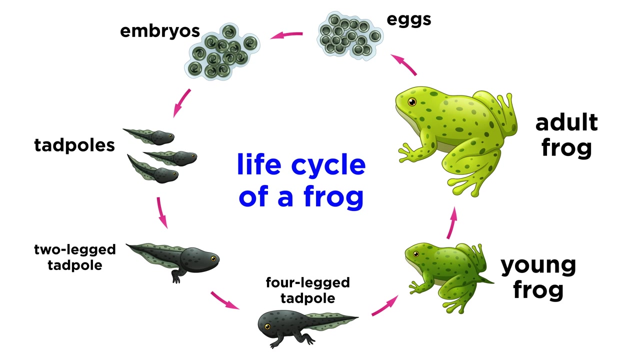 understanding of what ecologists study, starting at the most fundamental level: an organism. What can an ecologist study when it comes to a single organism? First, they can study an organism's life history or cycle. This pertains to how the organism grows, develops with time. 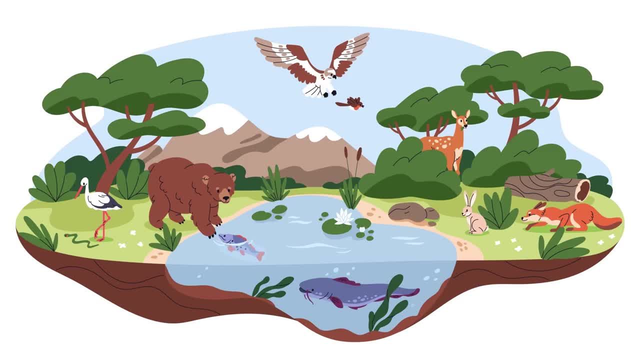 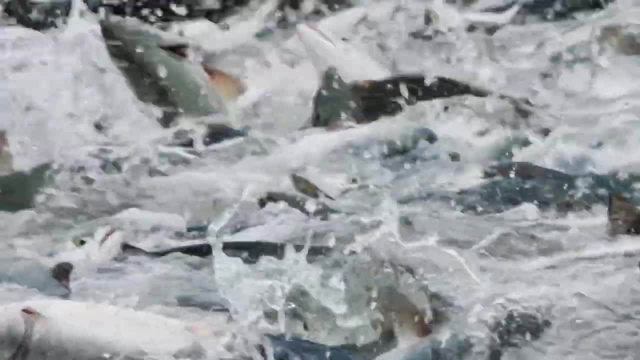 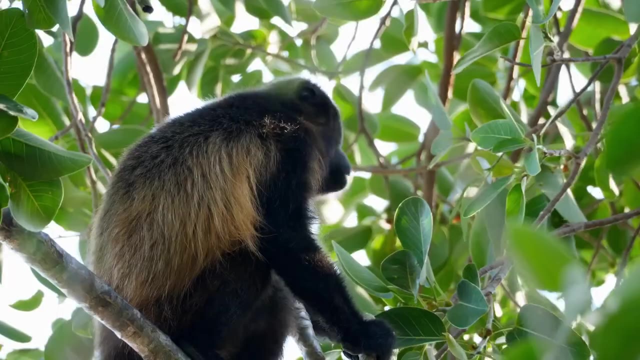 reproduces and ultimately survives. Life histories vary tremendously from one species to the next. For example, some organisms die immediately after reproducing, such as salmon, many insects and all grain crops, while others live on to reproduce repeatedly, Like most plants and vertebrates. Why is there so much variation? Researchers who study ecology. 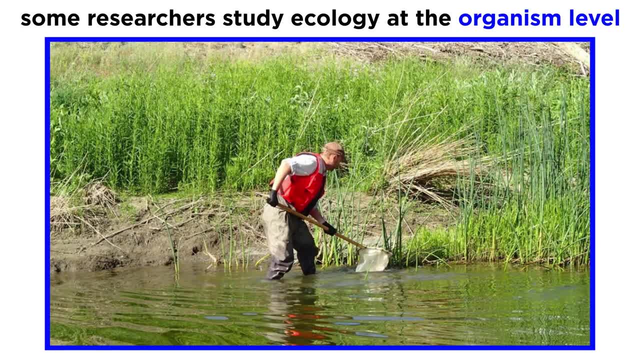 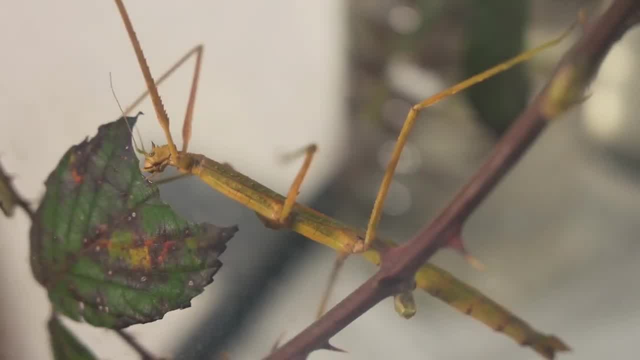 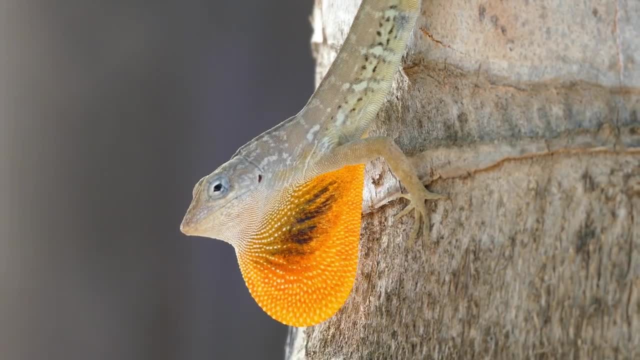 at the organism level, ask this question and many others like: how have different life cycles developed? How do they serve the organism? They also attempt to understand adaptations they observe in an organism. These are beneficial features or behaviors arising by natural selection which allow organisms to thrive in specific habitats. 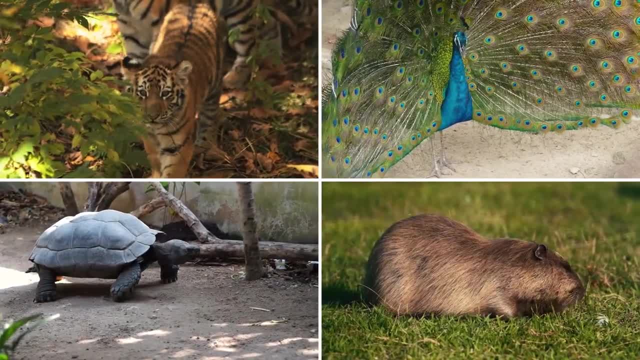 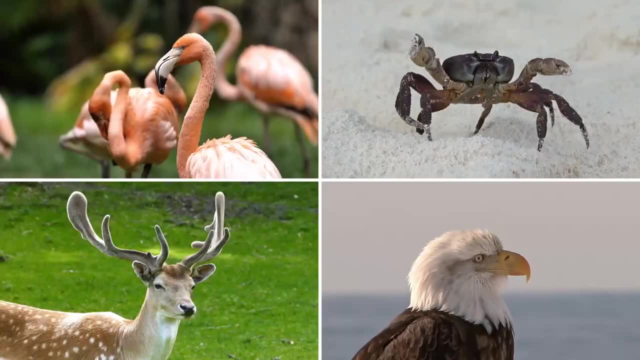 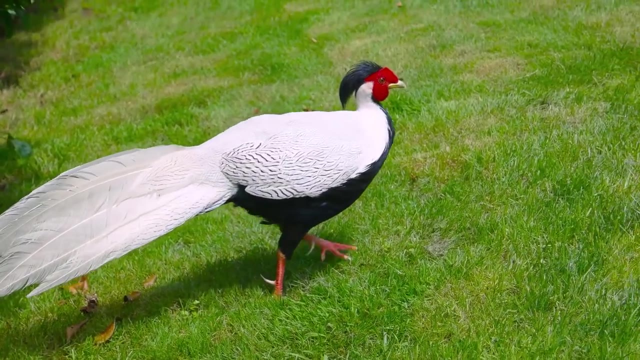 From varying body coverings like fur, feathers and scales, to patterns of color and camouflage, to defenses like a skunk's spray and a snake's venom, and finally to body parts like beaks, claws and antlers. Adaptations can take multiple forms, including: 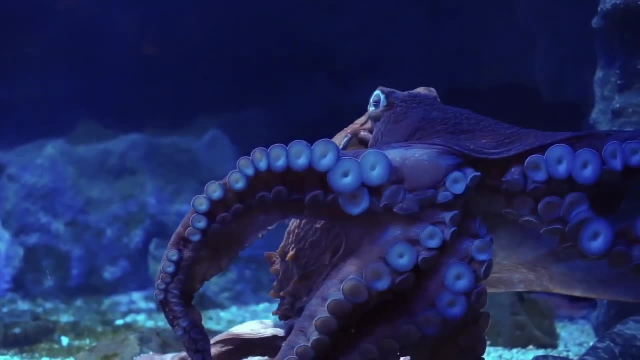 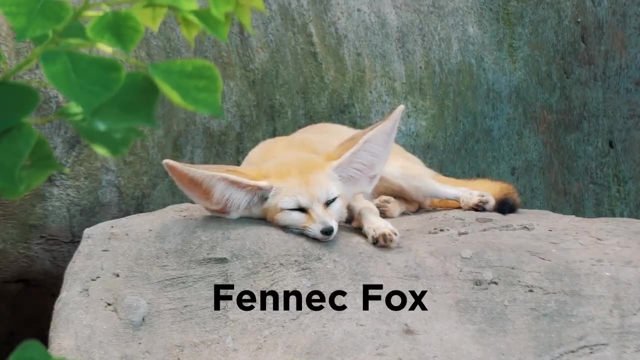 alterations to an organism's morphology, which refers to a structural change which gives an organism a greater chance of survival in its particular habitat. A great example is the fennec fox, which lives in the desert. It has large ears. You might think it's so, the fox. 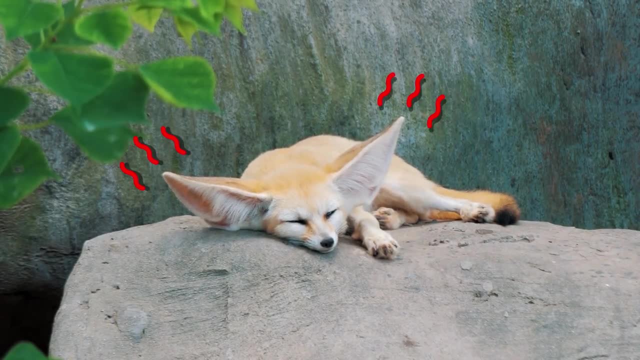 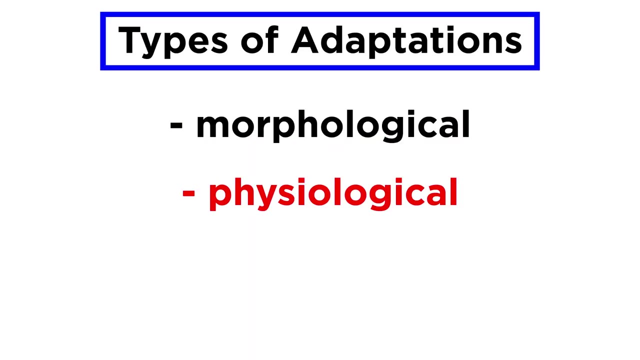 can hear better, but it's actually to allow heat to radiate away from the body, helping to cool the fox down in the intensely hot environment. Adaptations can be physiological in nature as well. These are internal processes that regulate and maintain homeostasis so that an organism is 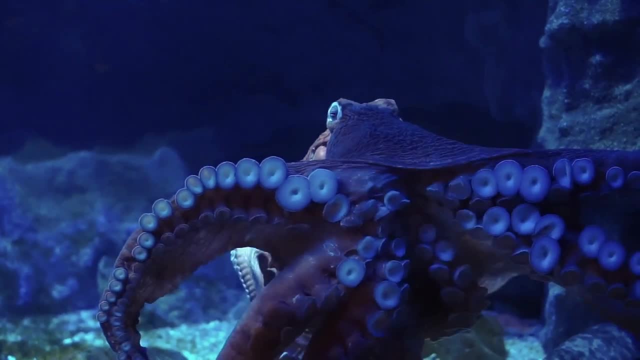 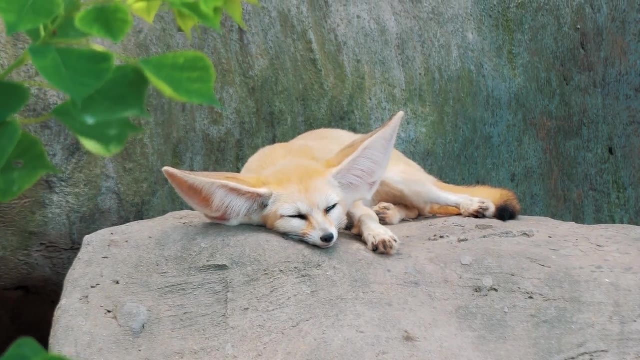 morphology, which refers to a structural change which gives an organism a greater chance of survival in its particular habitat. A great example is the fennec fox. It has a jullie, which is a species of pupus, that's especially, which lives in the desert. It has large ears, You might think it's, so the fox can hear better. 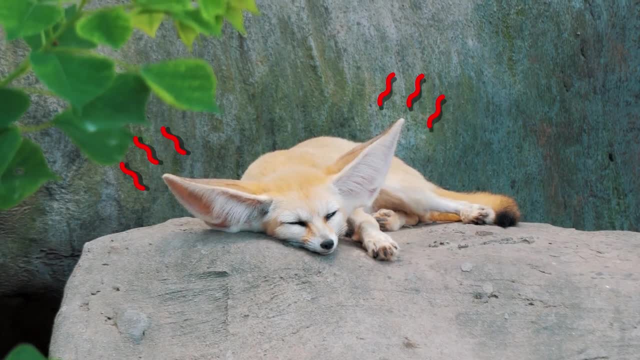 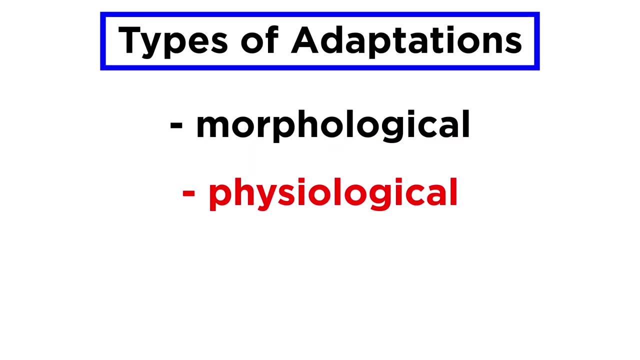 but it's actually to allow heat to radiate away from the body, helping to cool the fox down in the intensely hot environment. Adaptations can be physiological in nature as well. these are internal processes that regulate and maintain homeostasis so that an organism is able to. 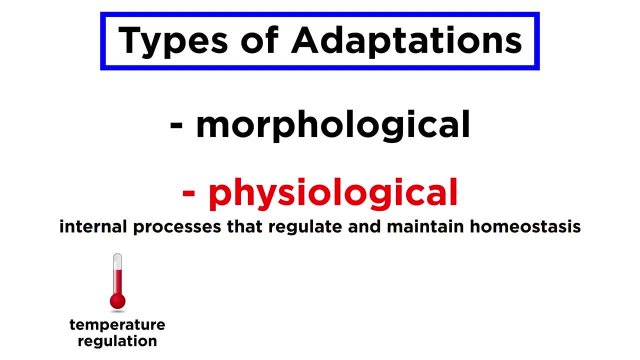 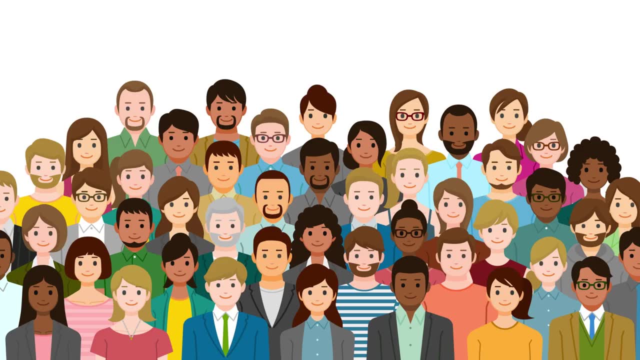 survive in the environment in which it exists. Examples of this include temperature regulation, release of toxins or poisons for protection, and even releasing natural antifreeze in the form of proteins to avoid freezing in cold environments. When it comes to humans, we can find some familiar examples. Calluses on our hands can be considered physiological. 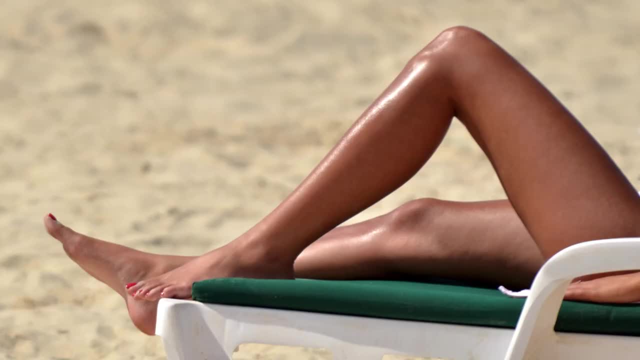 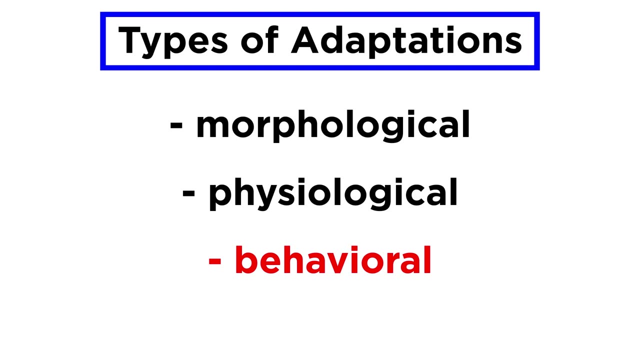 adaptations to repeated contact or pressure, as can tanning or darkening of the skin after repeated exposure to the sun. There are also behavioral adaptations, which are changes in behavior that certain organisms or species use to survive in their environment. There are two types. 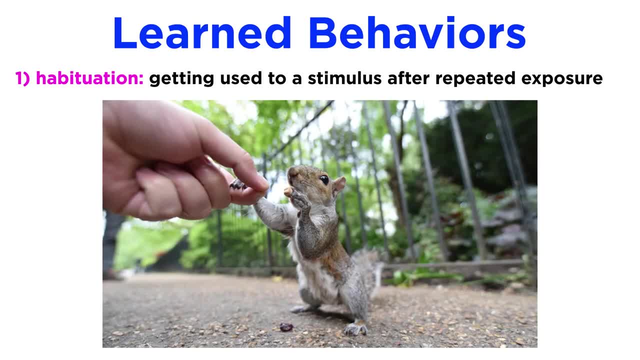 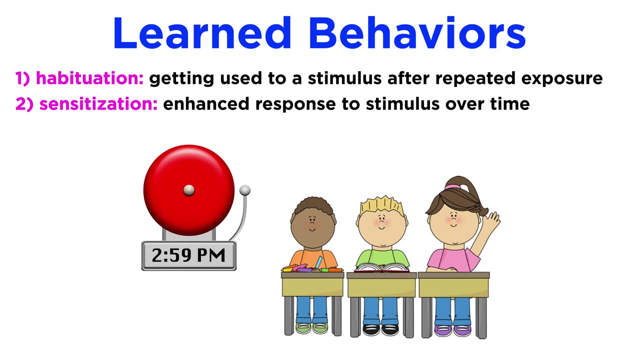 learned behaviors and instinctive behaviors. Learned behaviors include habituation, or getting used to a particular stimulus after being exposed to it multiple times, And sensitization, or responding to certain stimuli in an enhanced or more reactive manner. Think about becoming allergic to something like a certain type of food or pollen. 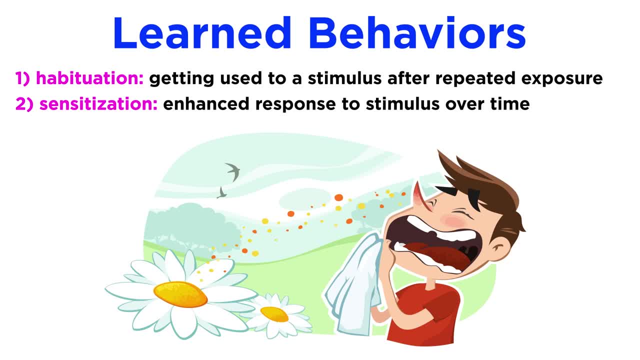 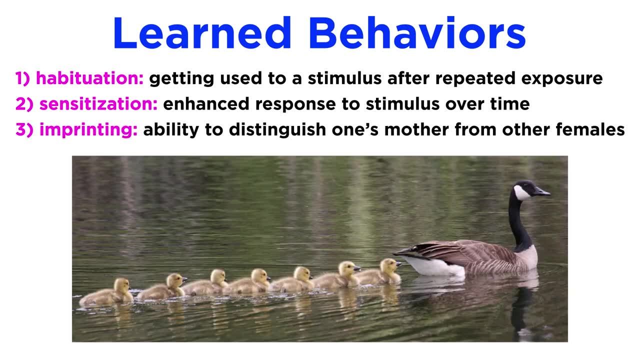 Your body, by becoming more sensitive, protects you from exposing yourself to these irritants in the future by producing a noticeable and worsening response. Then there's imprinting, an adaptive function that allows a young animal to distinguish its own mother from other females of. 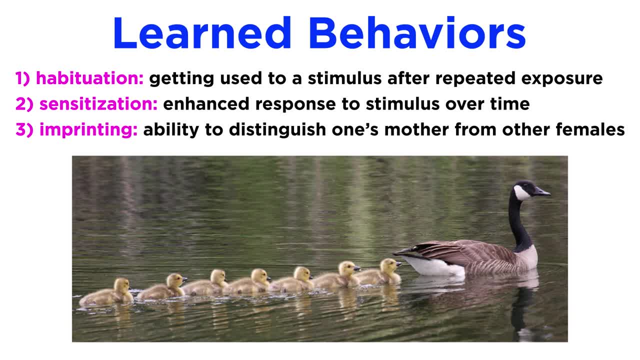 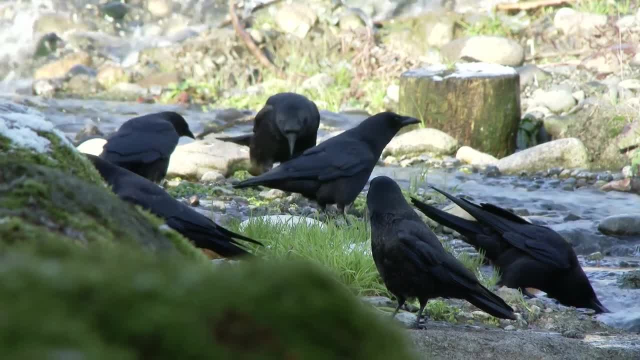 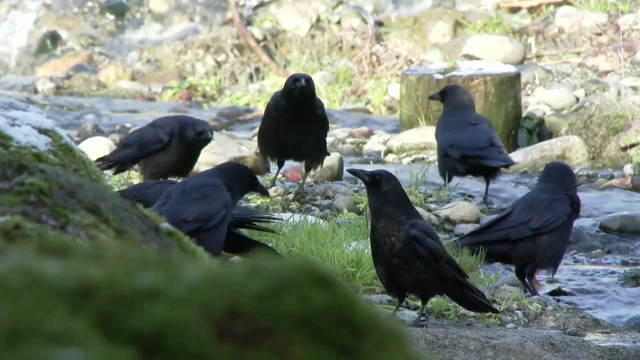 the same or different species and to remain near her for safety and protection. Learned behaviors can also come about from play and observation. Crows, for example, are notorious for their knack for observation-based learned behaviors, including solving puzzles and using tools. 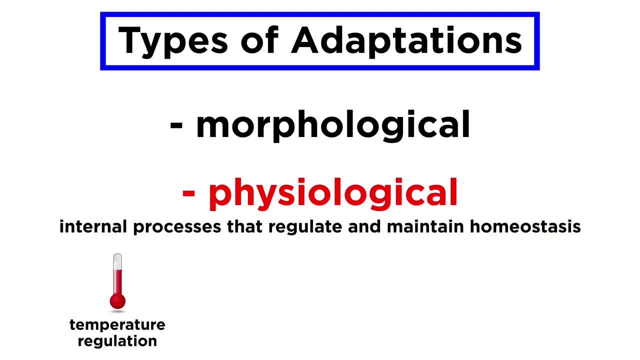 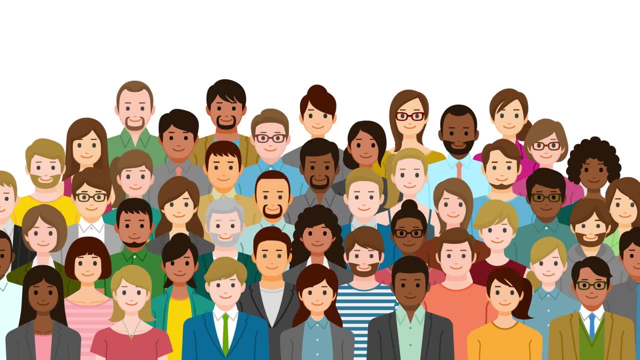 able to survive in the environment in which it exists. Examples of this include temperature regulation, release of toxins or poisons for protection, and even releasing natural antifreeze in the form of proteins to avoid freezing in cold environments. When it comes to humans, we can find some familiar examples. Calluses on our hands can. 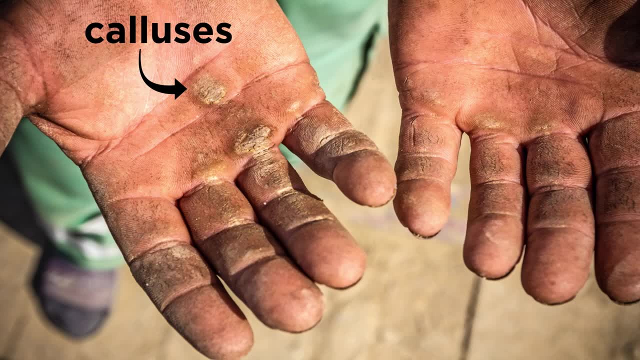 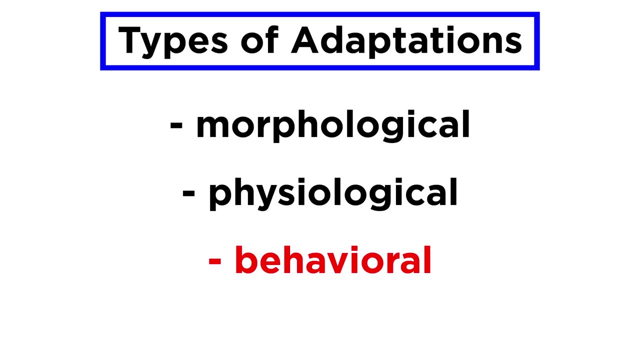 be considered physiological adaptations to repeated contact or pressure, as can tanning or darkening of the skin after repeated exposure to the sun. There are also behavioral adaptations, which are changes in behavior that certain organisms or species use to survive in their environment. There are two types: learned behaviors and instinctive behaviors. Learned 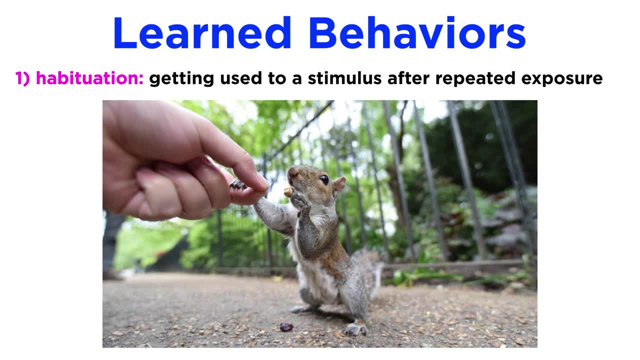 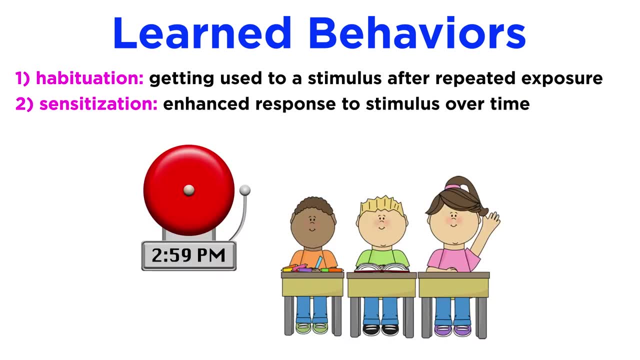 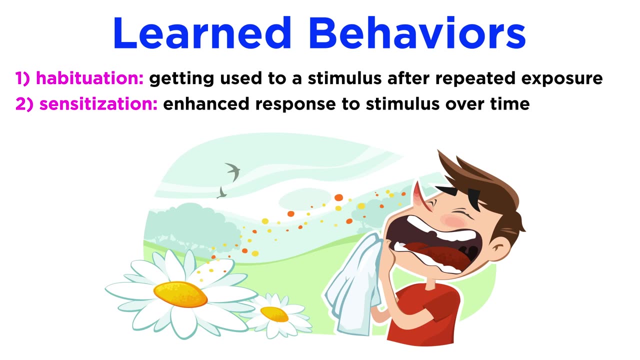 behaviors include habituation, or getting used to a particular stimulus after being exposed to it multiple times, And sensitization, or responding to certain stimuli in an enhanced or more reactive manner. Think about becoming allergic to something like a certain type of food or pollen. Your body, by becoming more sensitive, protects you from exposing. 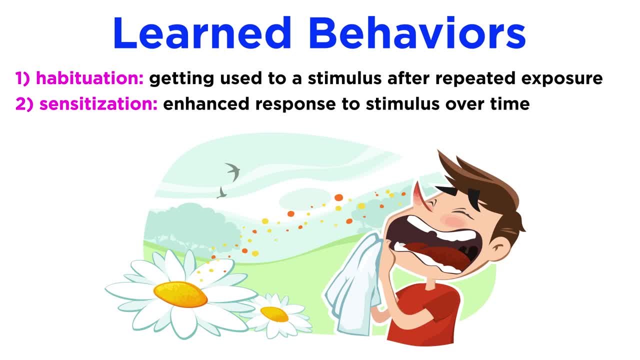 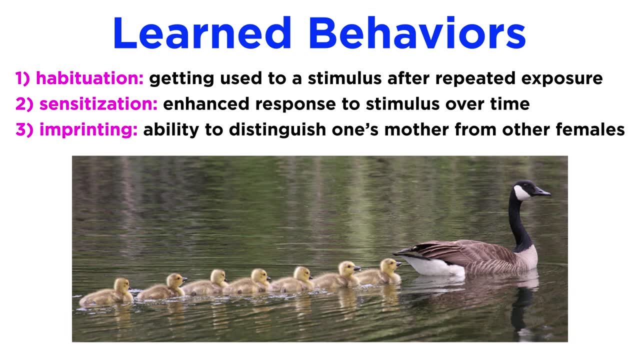 yourself to these irritants in the future by producing a noticeable and worsening response. Then there's imprinting, an adaptive function that allows a young animal to distinguish its own mother from other females of the same or different species and to remain near her for safety and protection. Learned behaviors can also come about from play and observation. 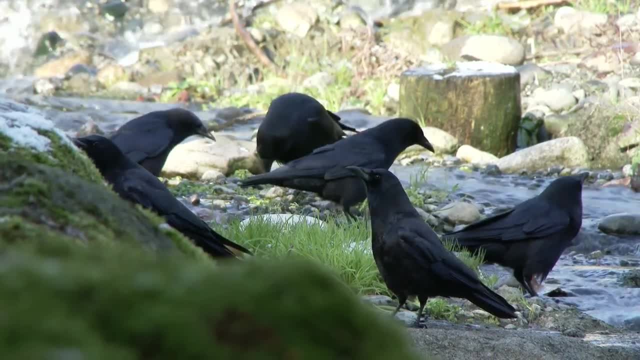 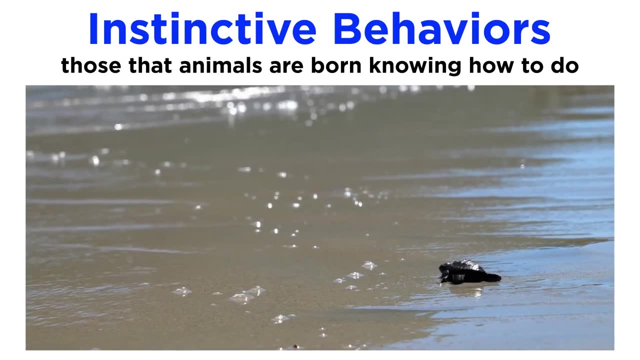 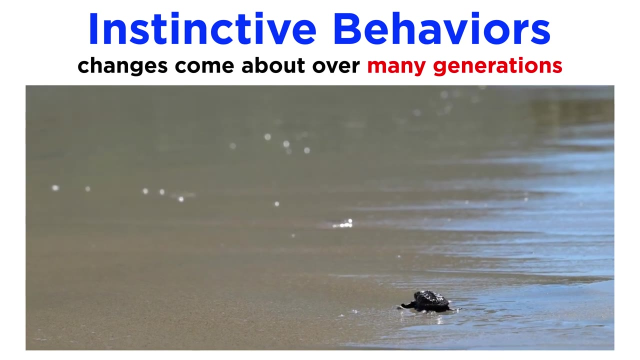 Crows, for example, are notorious for their instinctive behavior. Crows, for example, are notorious for their knack for observation-based learned behaviors, including solving puzzles and using tools. Instinctive behaviors are those behaviors that animals are born knowing how to do. Changes usually come about over many generations until they finally become. 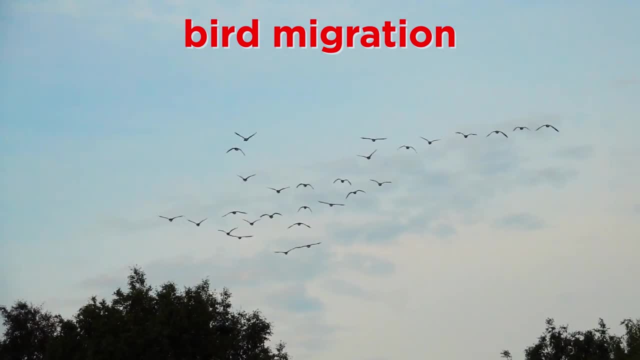 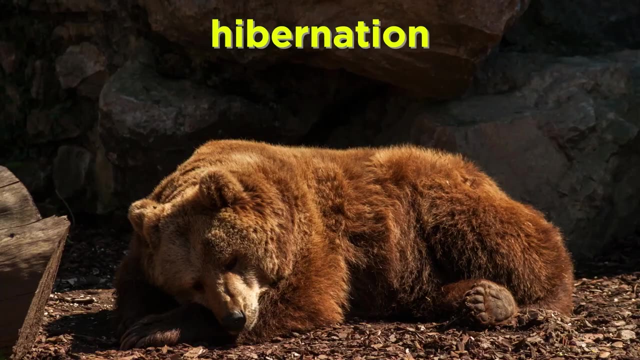 a part of instinctive behavior. Some examples include the migration of birds like geese during the cold seasons of the year to areas further south in search of food. The hibernation of some mammal-like animals can also be a part of instinctive behavior. Some examples include the migration of birds like geese during the cold seasons of the year to areas further south in search of food. The hibernation of some mammals. 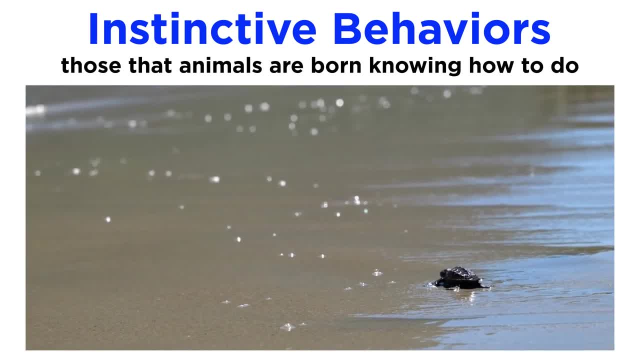 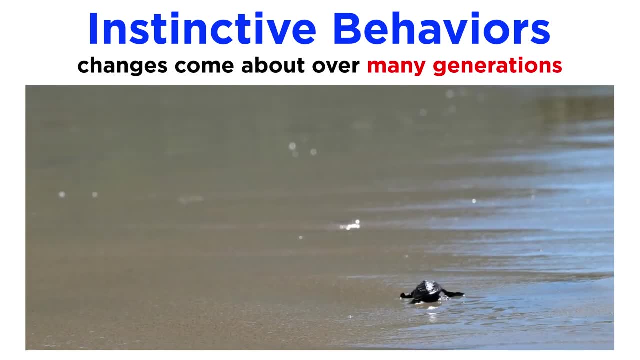 Instinctive behaviors are those behaviors that animals are born knowing how to do. Changes usually come about over many generations until they finally become a part of instinctive behavior. Some examples include the migration of birds like geese during the cold seasons of the year. 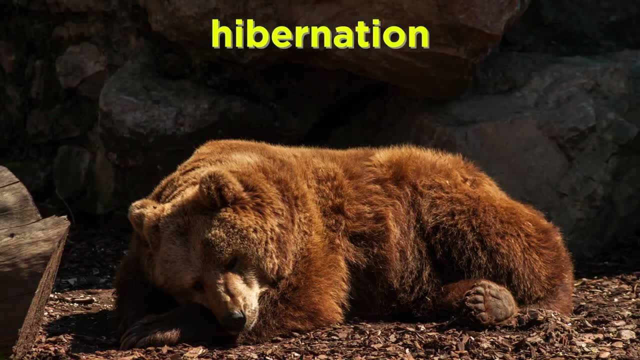 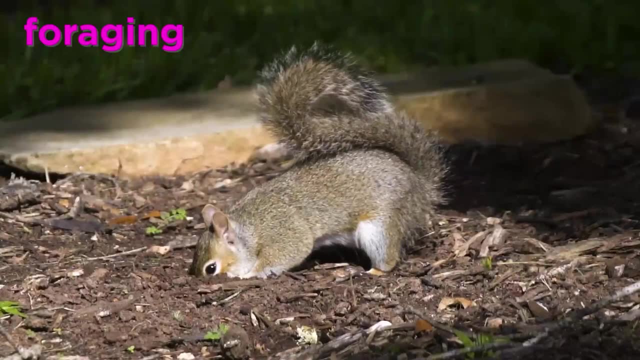 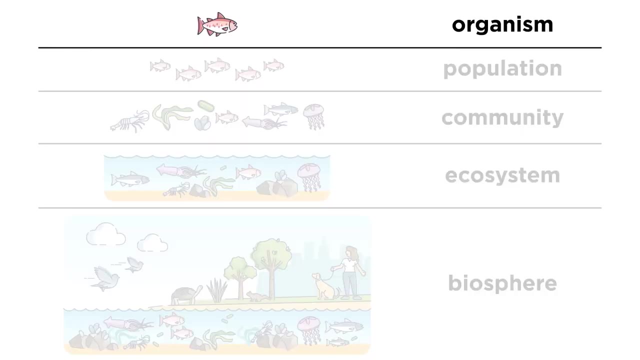 to areas further south in search of food. The hibernation of some mammals during the winter, like bears. Courtship or mating patterns And foraging behaviors, which include knowing ways of finding food depending on the habitat or environment, Moving on from organisms. 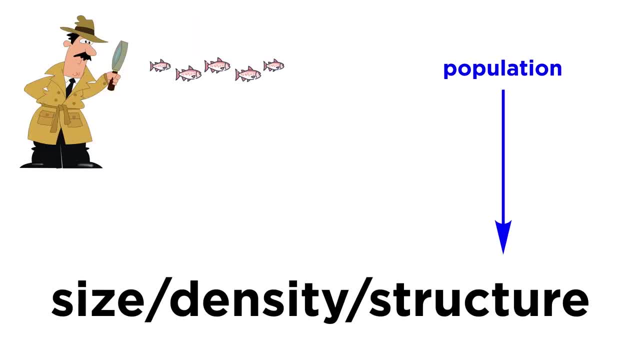 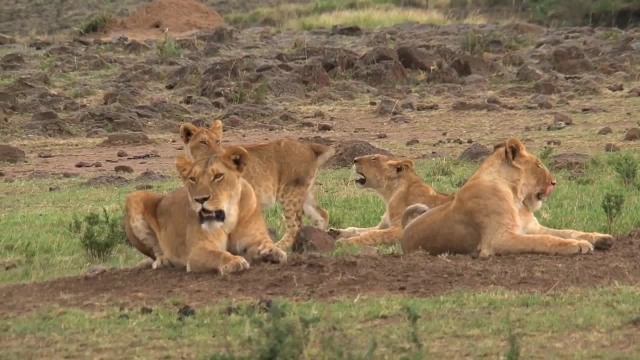 population ecologists are scientists who study the size or total number of individuals, as well as density and structure of populations and how they change. Of interest are a population's geographic range, which has limits that a species can tolerate, like fluctuations in temperature or moisture. The study of population ecology also includes 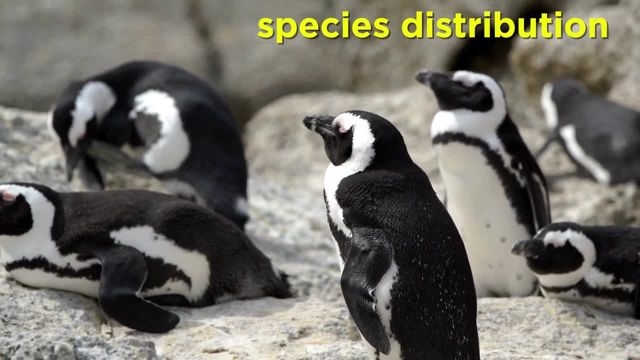 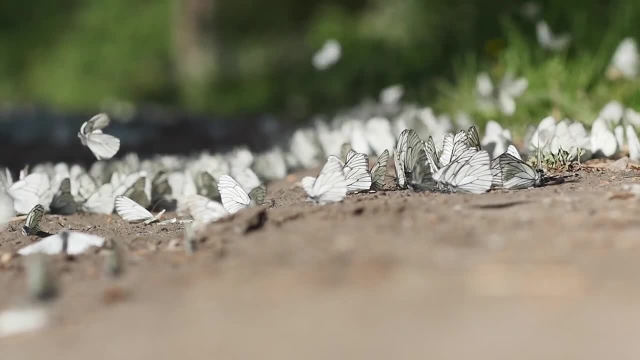 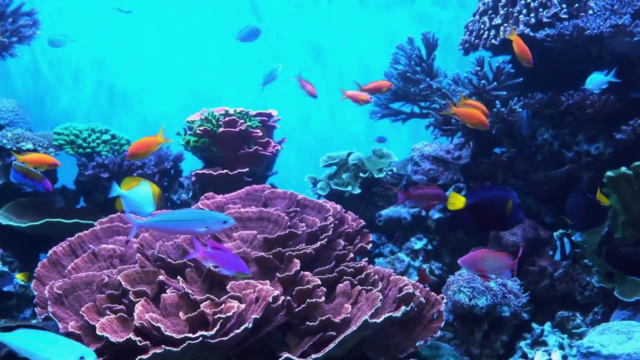 understanding, explaining and predicting species distributions? Why do species inhabit particular areas and how are they prevented from establishing beyond their range limits? Such range questions have become popular in the last decade or so in response to concerns about climate change. Additionally, what are the birth and death rates of a particular? 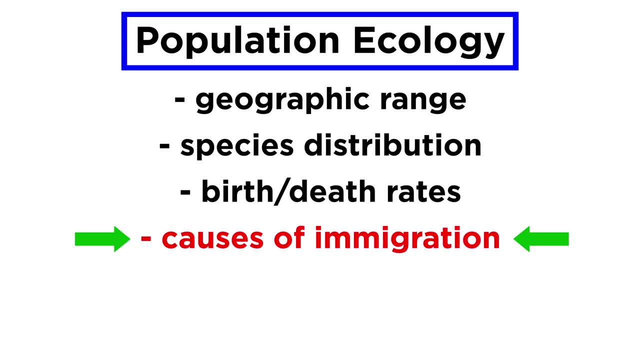 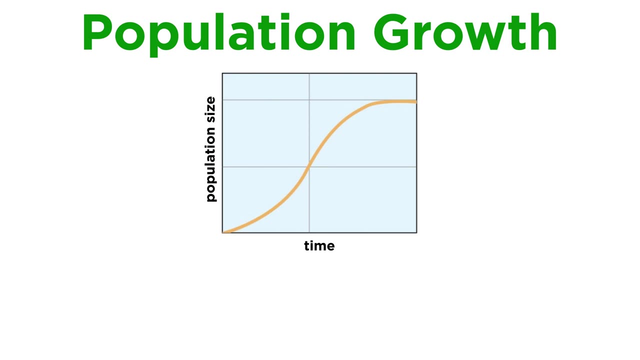 species. What urges populations to immigrate or explore new areas beyond their previous range? What causes them to emigrate when they leave familiar territory altogether? What are the long-term probabilities of species persisting and surviving in certain habitats? What factors play a role in deciding this? Now let's discuss population. 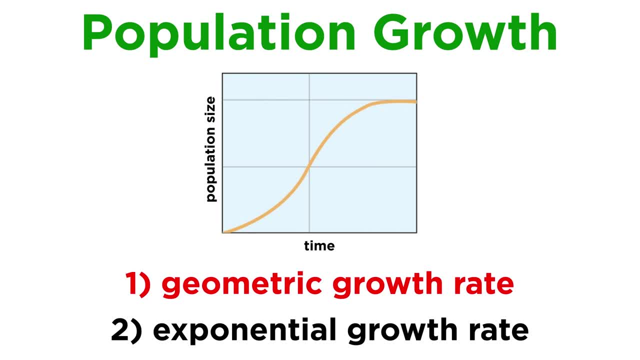 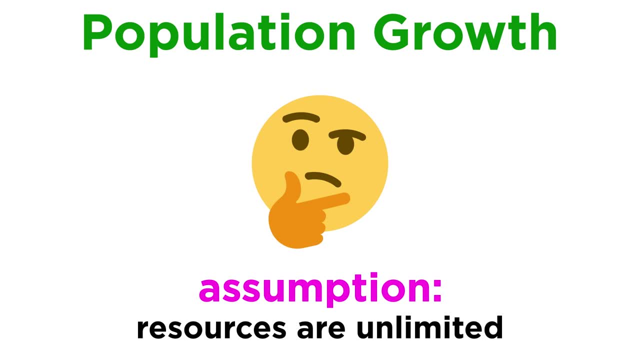 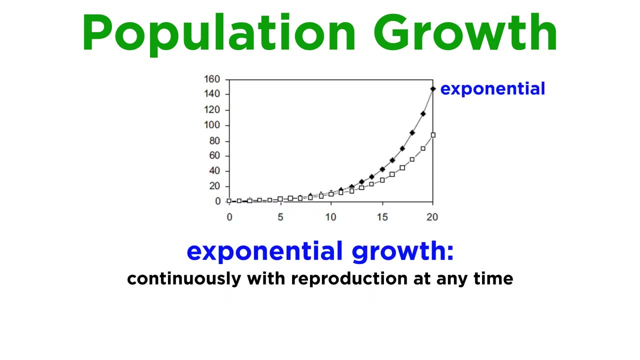 growth. Populations can grow in two different modes: at geometric rates or at exponential rates. While exploring these, keep in mind that we will be assuming the presence of unlimited resources which urge population growth. Exponential growth happens continuously, with reproduction happening at any time, like in human populations. Geometric populations: 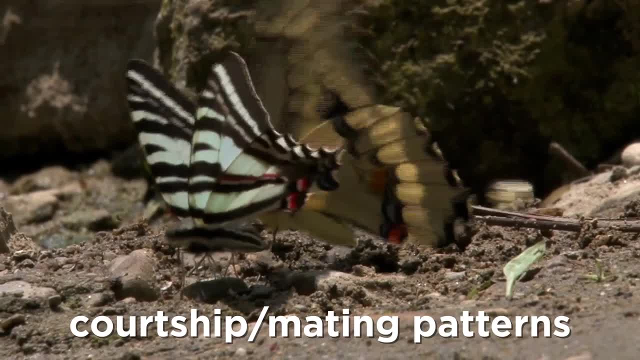 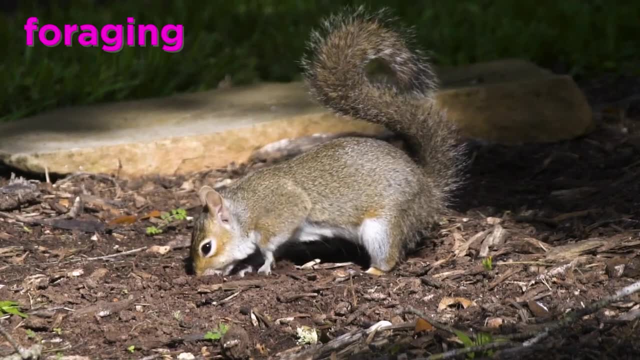 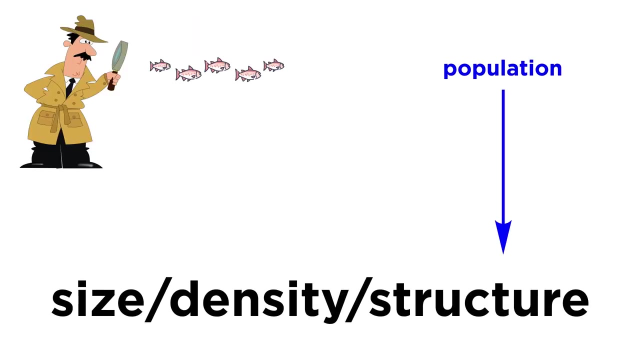 during the winter, like bears, Courtship or mating patterns And foraging behaviors, which include knowing ways of finding food depending on the habitat or environment. Moving on from organisms, population ecologists are scientists who study the size or total number of individuals, as well as density and structure of populations and how they 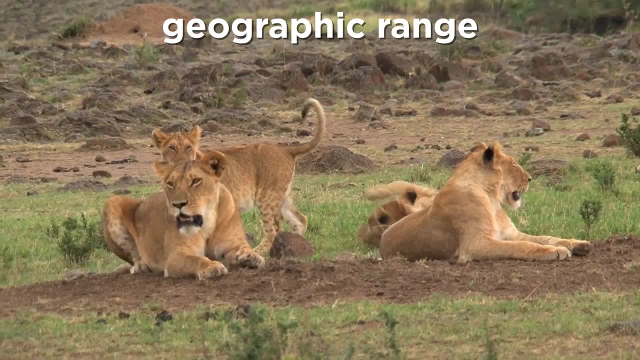 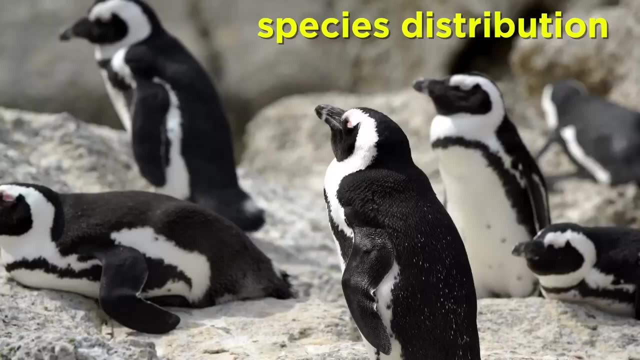 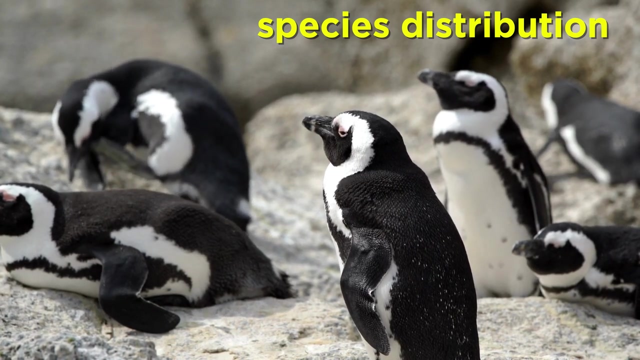 change over time. Of interest are a population's geographic range, which is the size of a population, which has limits that a species can tolerate, like fluctuations in temperature or moisture. The study of population ecology also includes understanding, explaining and predicting species distributions. Why do species inhabit particular areas and how are they prevented? 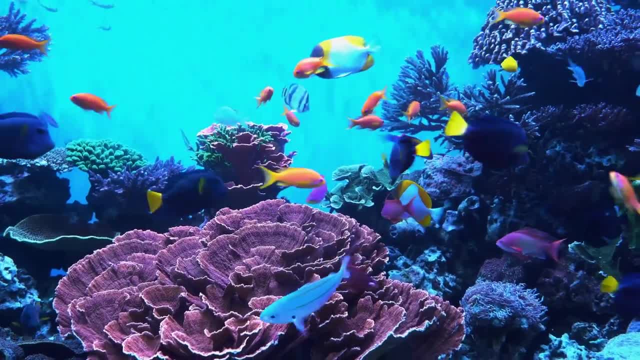 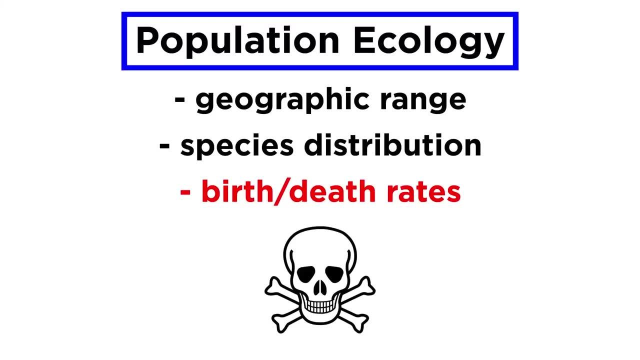 from establishing beyond their range limits. Such range questions have become popular in the last decade or so in response to concerns about climate change. Additionally, what are the birth and death rates of a particular species? How does a species change over time? What causes populations to emigrate or explore new areas beyond their previous range? What? 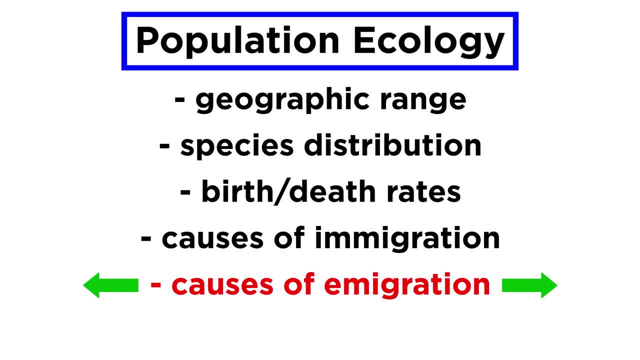 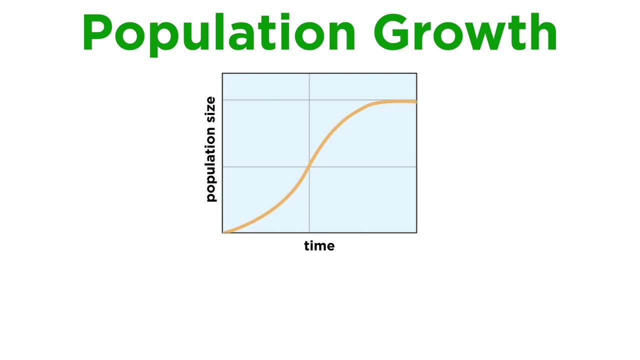 causes them to emigrate when they leave familiar territory altogether? What are the long-term probabilities of species persisting and surviving in certain habitats? What factors play a role in deciding this? Now let's discuss population growth. Populations can grow in two different modes. at geometric, 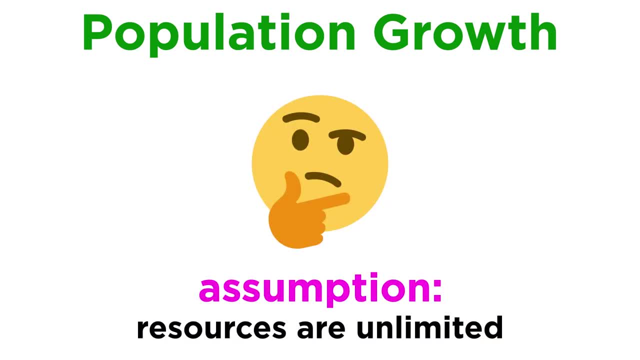 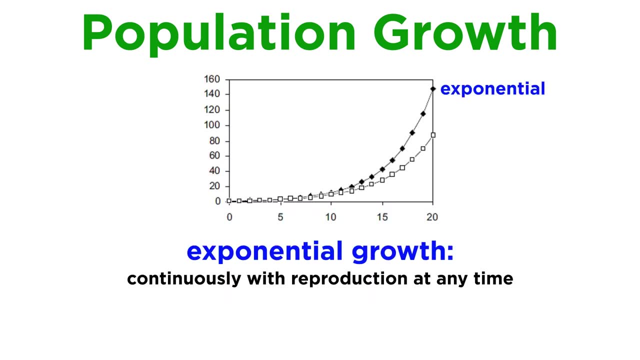 rates or at exponential rates. While exploring these, keep in mind that we will be assuming the presence of unlimited resources which urge population growth. Exponential growth happens continuously, with reproduction happening at any time. like in human populations, Geometric populations grow through pulsed reproduction instead. An example of this is deer, which 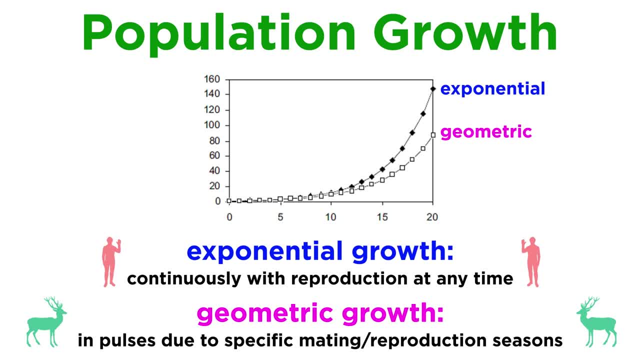 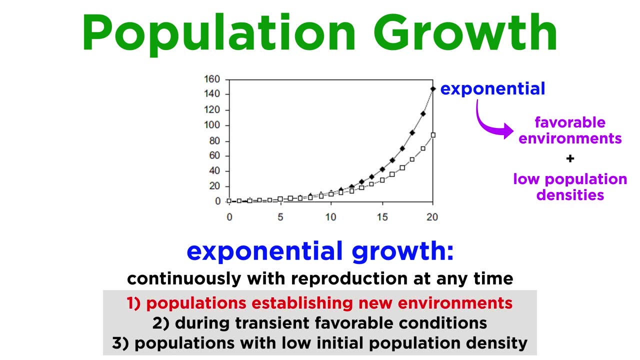 have a constrained mating and reproduction season, keeping them from constantly reproducing. When exponential growth occurs, it is in favorable environments and at low population densities. Because of this, exponential growth may apply to populations establishing new environments during transient favorable conditions and by populations with low initial population. 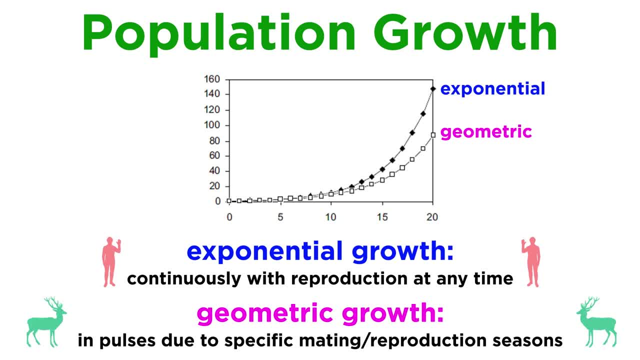 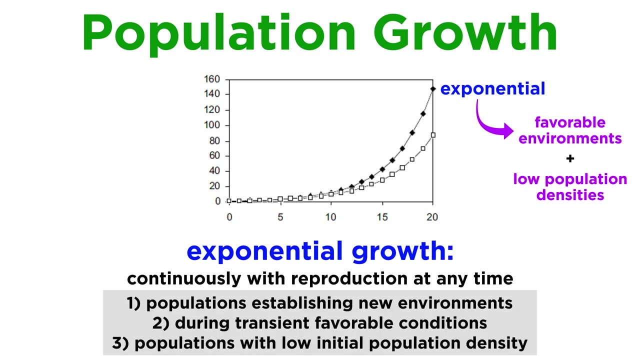 grow through pulsed reproduction instead. An example of this is deer, which have a constrained mating and reproduction season, keeping them from constantly reproducing. When exponential growth occurs, it is in favorable environments and at low population densities. Because of this, exponential growth may apply to populations establishing new environments during transient. 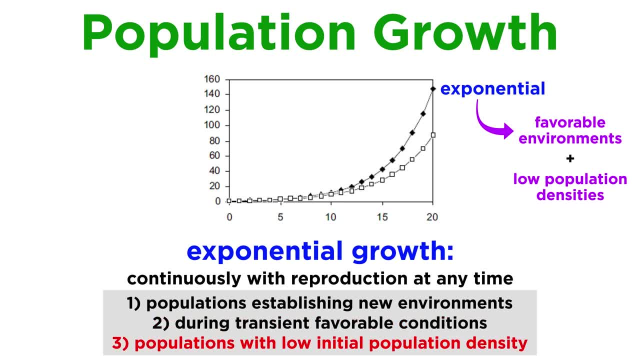 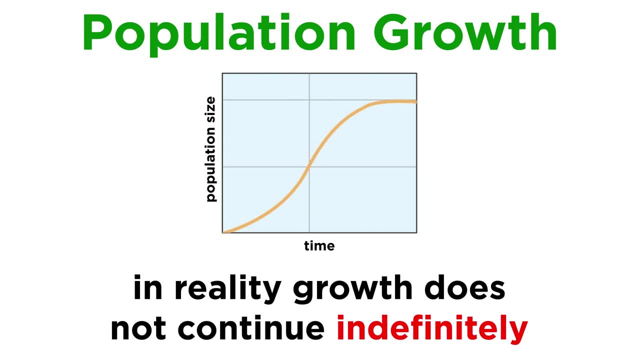 favorable conditions and by populations with low initial population density. Of course, neither geometric nor exponential growth can continue indefinitely In nature. population growth must eventually slow and population size eventually ceases to increase. As resources are depleted, the population growth rate slows and eventually stops. 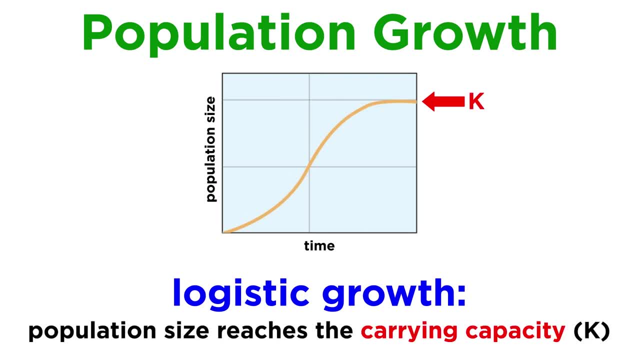 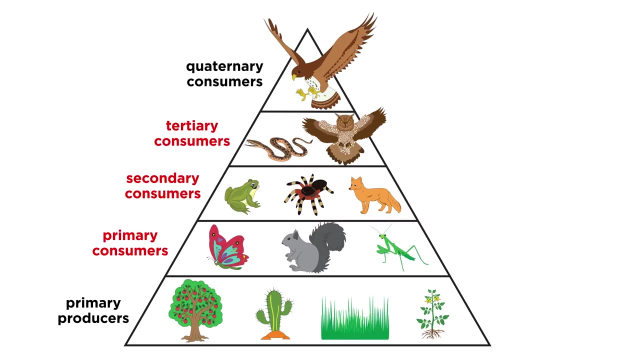 This is known as logistic growth. The population size at which growth stops is generally called the carrying capacity, which is the number of individuals of a particular population that the environment can carry or support. Carrying capacity is characterized by equal death rates, creating a population growth of zero In some populations, organisms in lower 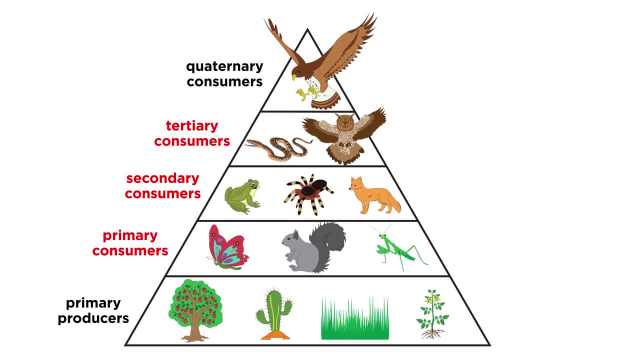 trophic levels, meaning the positions that organisms occupy in a food web, are controlled by organisms at the top. This is known as top-down control. For example, carnivores at the top keep the herbivore population in check. If herbivores weren't controlled, all the plants 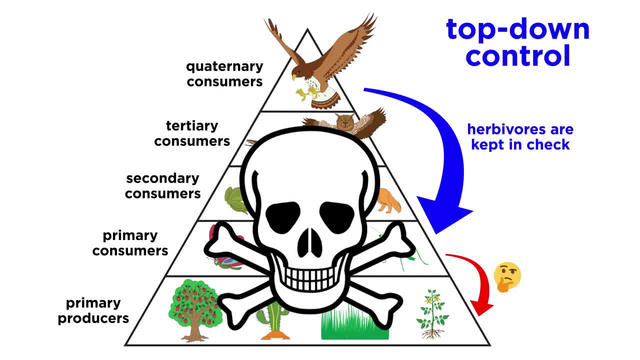 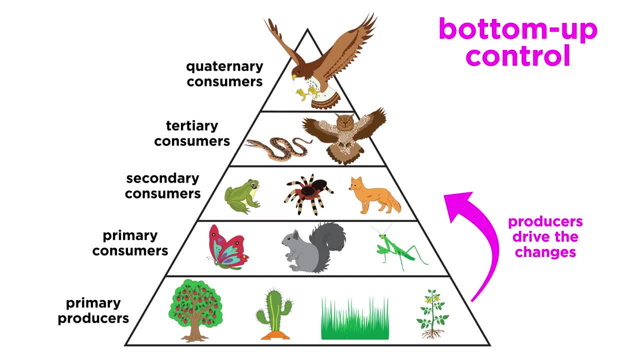 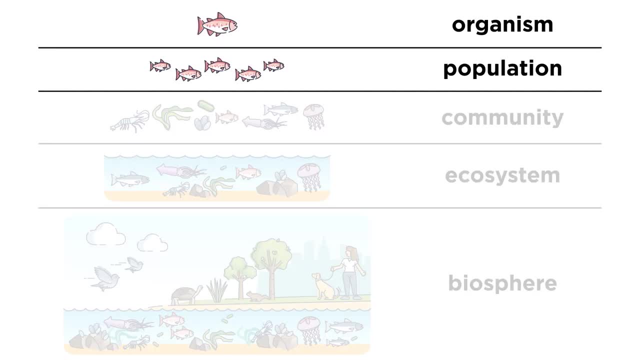 would be eaten, leading to a potential collapse of the entire ecosystem. In bottom-up control, it's the producers at the lower trophic levels who drive the changes. instead. If plant populations change, then the population of all species will be impacted, With organisms and populations. 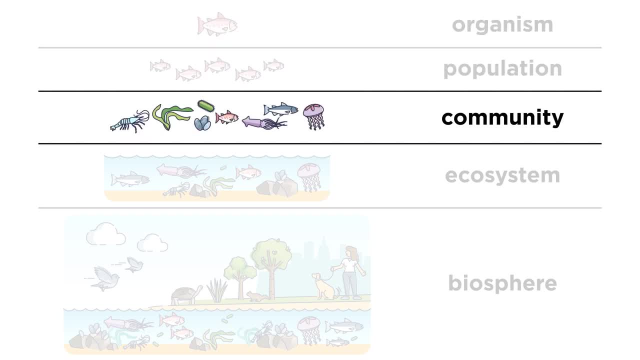 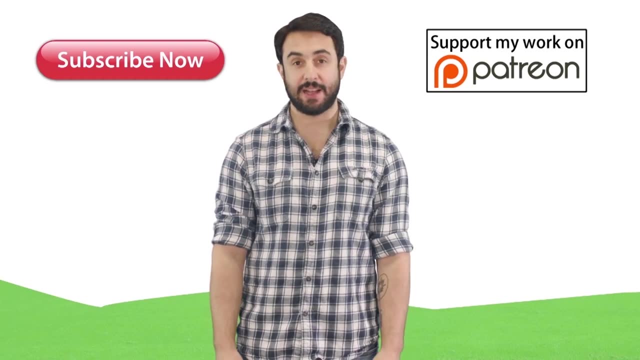 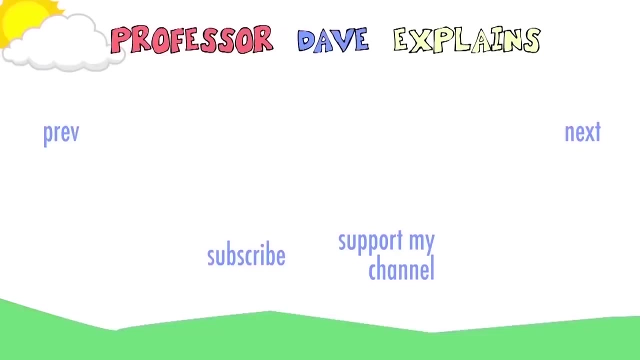 better understood. let's move forward and look at communities of organisms. Thank you for watching.